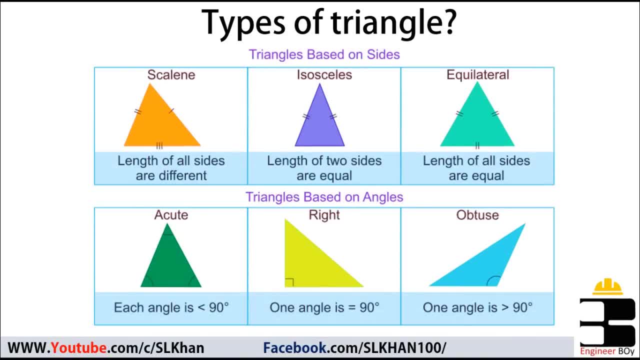 Triangles as you can see we got six types of triangles where three are based on sides and the 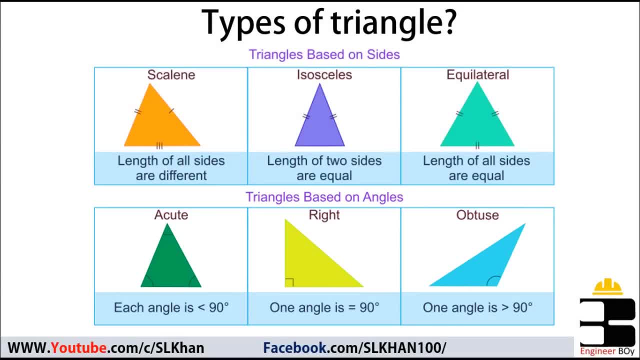 rest are based on angles. So just stop the video here and study the given table. As you can see 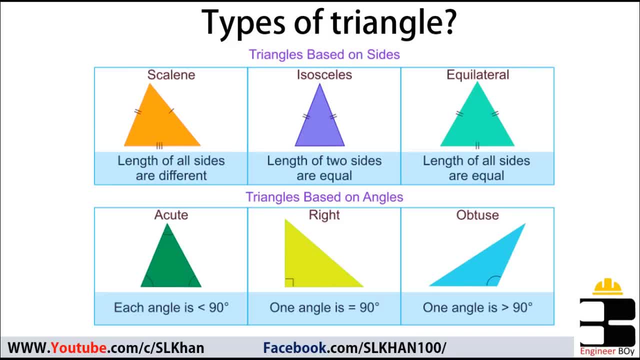 in based on sides we have skillen, isosceles and equilateral triangle and based on angles we got 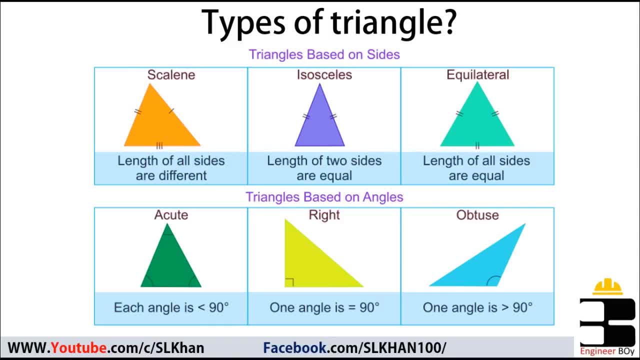 acute right angle triangle and obtuse triangle. I hope you already know all these things okay I 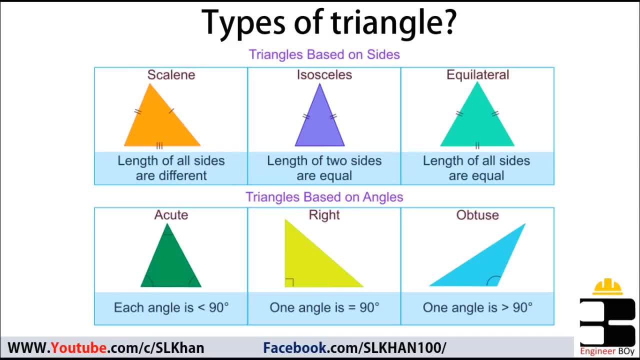 these six types of triangle so come directly into the area determination because in this video our 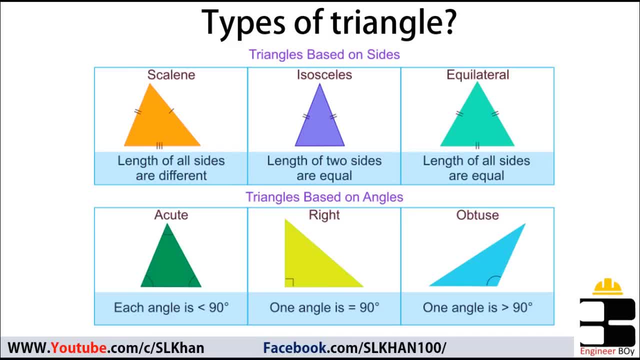 approach is about area all right so let's start with the basic one that's the right angle triangle 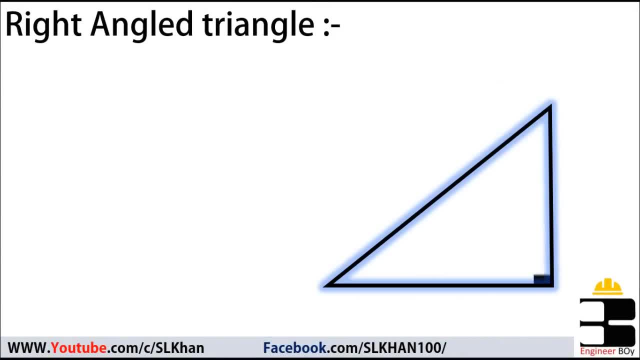 so the area of this triangle must be one half times base cross its perpendicular which is 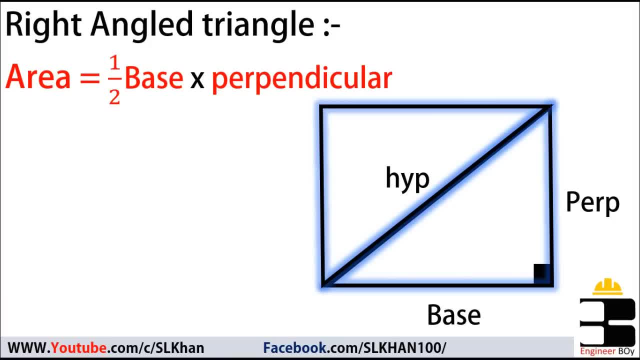 actually just half of the rectangle so whenever you have base and perpendicular of the triangle 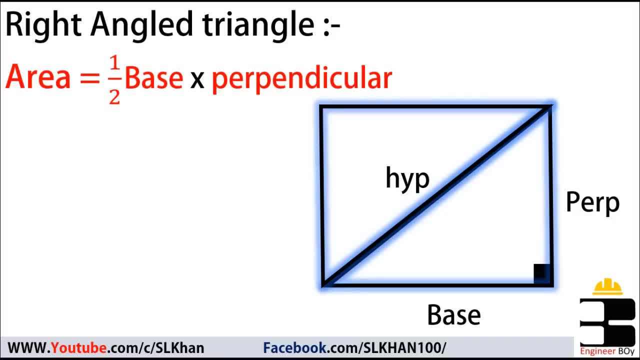 that is a right angle triangle you can use this simple formula to determine its area 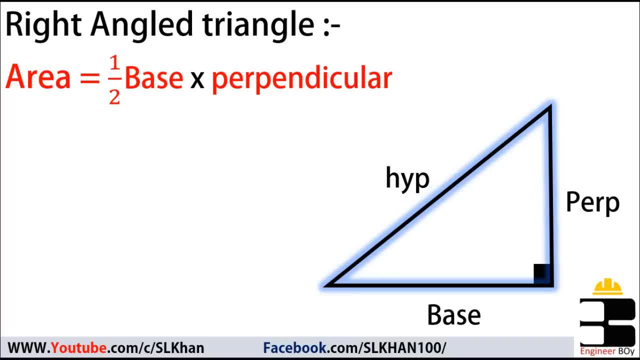 also if you don't have these two elements you can work them out from other elements by using 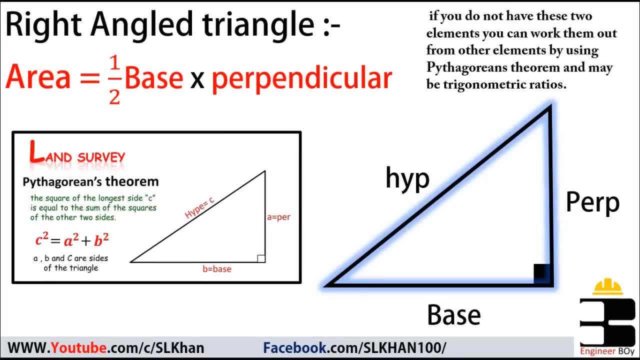 pythagorean theorem and maybe trigonometric ratios to learn pythagorean theorem in detail just go and watch it in the same channel link to that video is down below in the video description 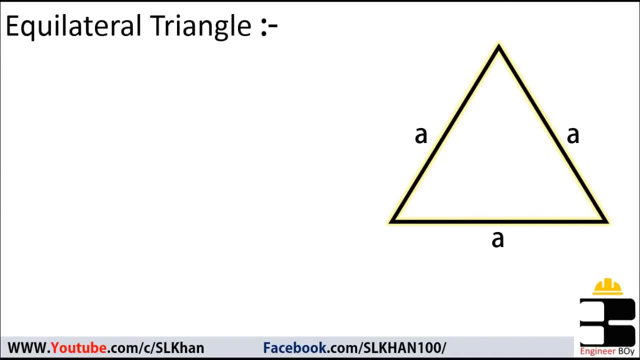 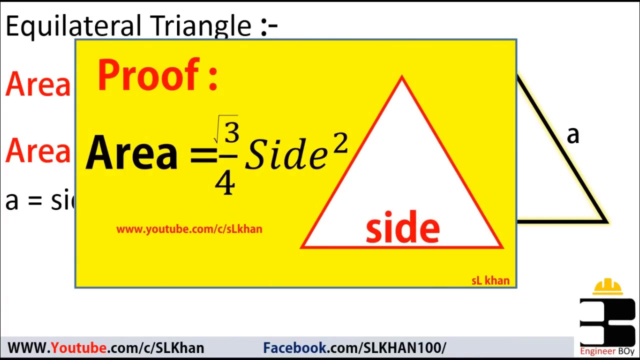 another one is an equilateral triangle has length of all sides equal that is just the definition of an equilateral triangle okay to determine the area of this triangle we can use this simple formula which is actually area equals square root 3 divided by 4 times a square or you can say 0.433 a square where a is just of course the side of the triangle the derivation to this formula is also been uploaded in the same channel 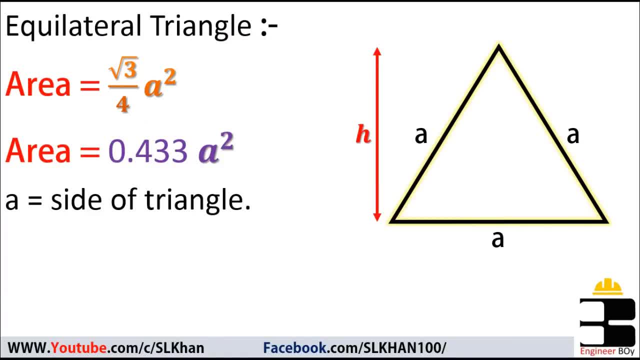 so if side of an equilateral triangle is known just use this simple formula however if it side isn't known and its perpendicular is known instead of it then you can use the same formula used by right angle triangle or you can also work out at side by using trigonometric ratios or trigonometric 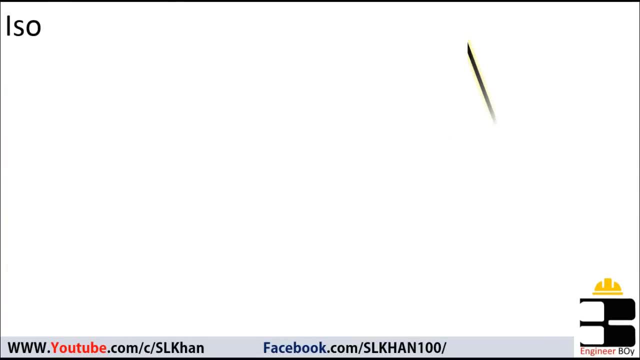 identities okay another one is an isosceles triangle which has length of two sides equal area is enough sample for example if you have sides of an isosceles triangle just work out its perpendicular by using pythagorean theorem and then determine its area by using the same formula used for right angle triangle so the area of an isosceles triangle is one half base times 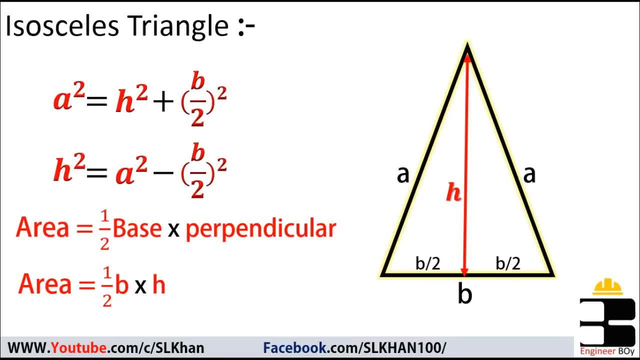 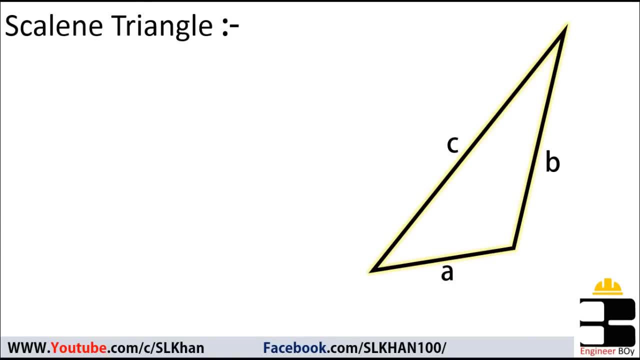 its perpendicular the final challenge we can face is the skill and triangle which has all sides different in length this can also be acute as well as obtuse triangle so the formula but this 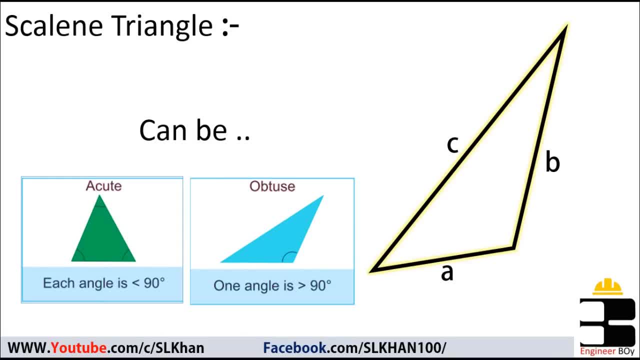 approach is going to be very important and the formula for this triangle can be used for all types of triangles so this is very important okay and that's of course hiros formula which is of course the area of any types of triangle equals square root is into s minus a times is minus b times is minus a 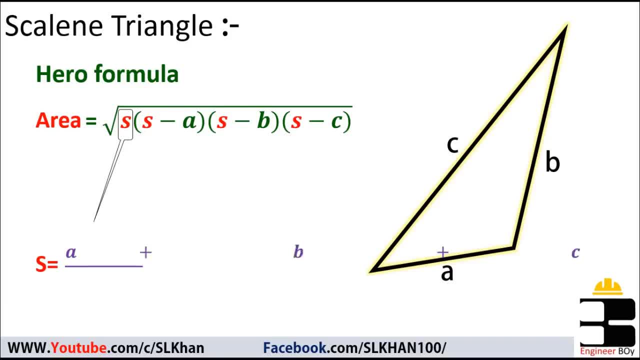 minus C where S is the semi-pyramidal of the triangle and ABC are the sides of triangle so 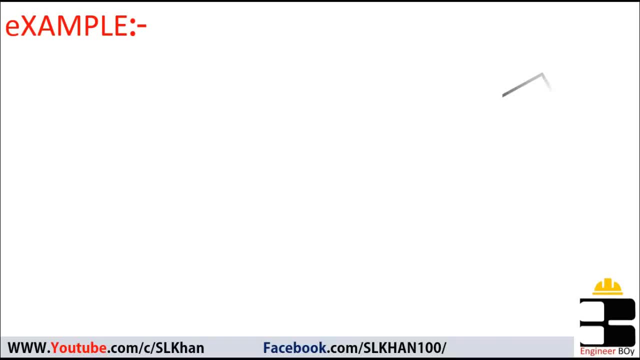 if we have learned something or not suppose if we are asked to find the area of the given property 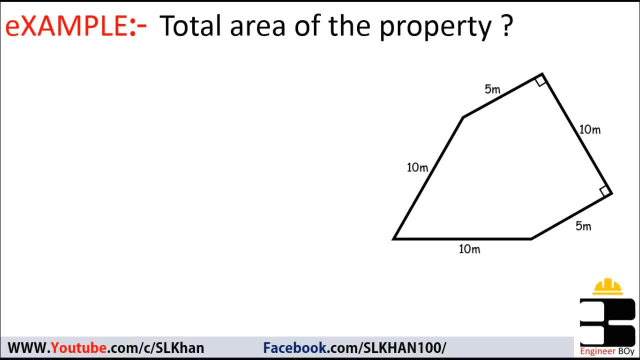 so how can we do that all right so let's come into the solution guess what I'm gonna do here is to split this property into two parts and I'm gonna draw a line just like that one okay 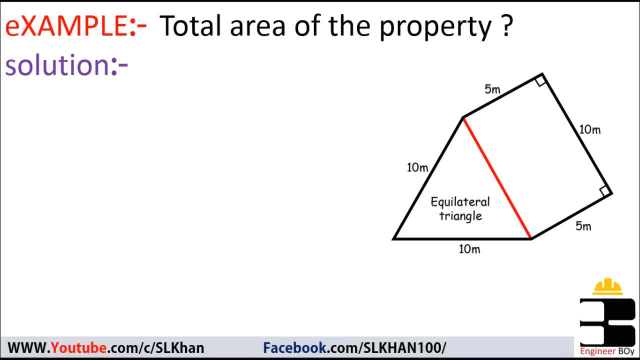 you can see that okay so here we got two shapes an equilateral triangle and a rectangle that means the total area of the property is going to be area of the triangle which is in equal 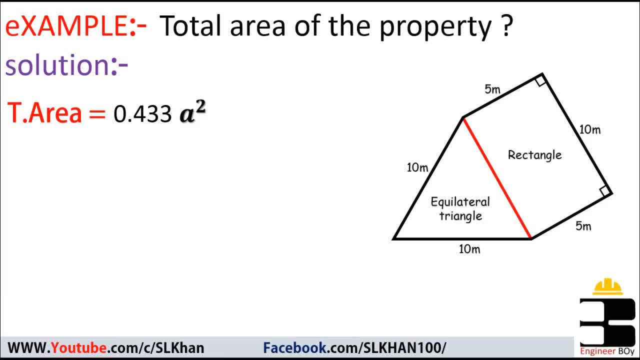 triangle and that is 0.433 a square plus area of the rectangle which is a cross b and these are the